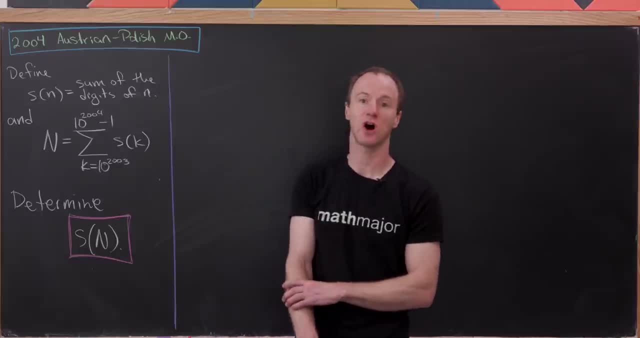 Today we're going to look at a pretty cool problem from the 2004 Austrian-Polish Math Olympiad. So there are a lot of moving parts here. but that being said, I think there are also a lot of nice techniques, And while it's kind of surprising at first glance that this problem 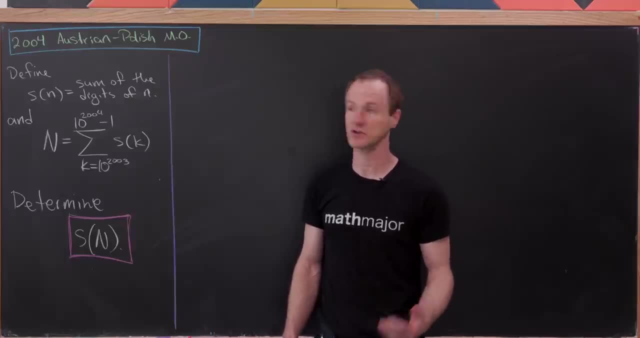 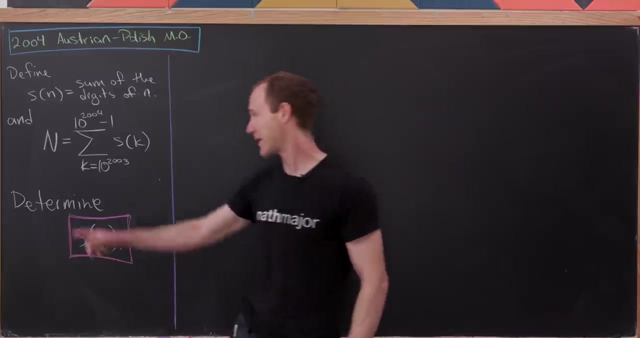 is even possible, although we'll see that it's fairly straightforward. Okay, so let's define s of n to be the sum of the digits of the natural number, n- I guess we should say here- expressed in base 10.. And then we'll set capital n equal to the sum as k goes from 10 to the 2003. 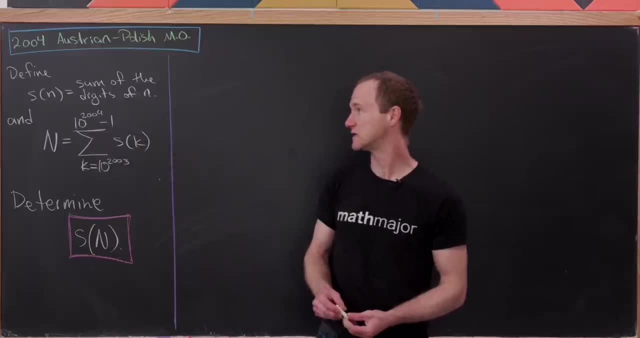 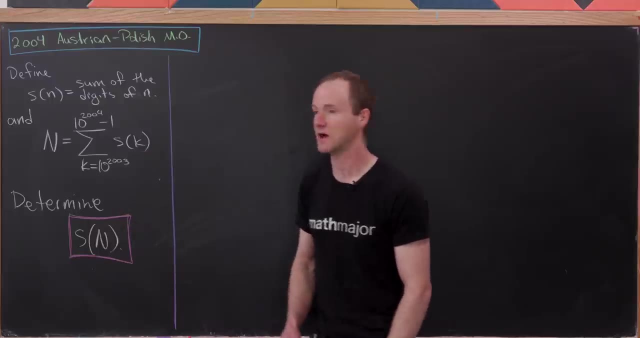 all the way to 10, to the 2004 minus 1 of s of k, And then our goal is to determine s of capital n. So we've got like really a composition of this function s with, well, maybe, the sum of values. 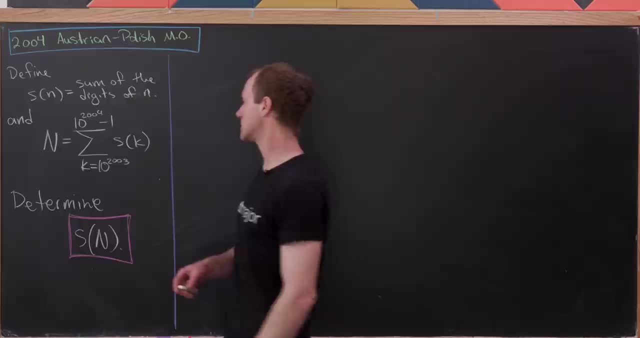 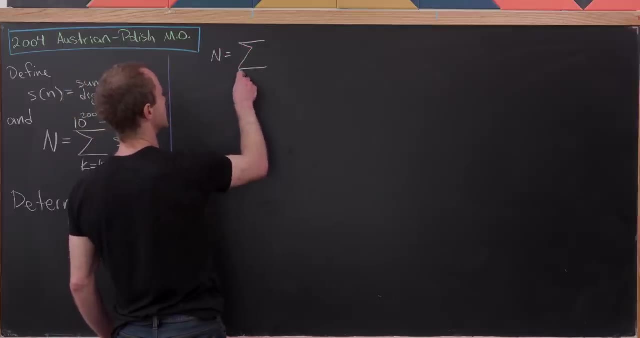 of s. So I think that's pretty interesting. Now let's start off by observing that n is really of this form. Notice it's equal to the sum, as k goes from 0 to this upper point. So 2004 minus 1 of s. 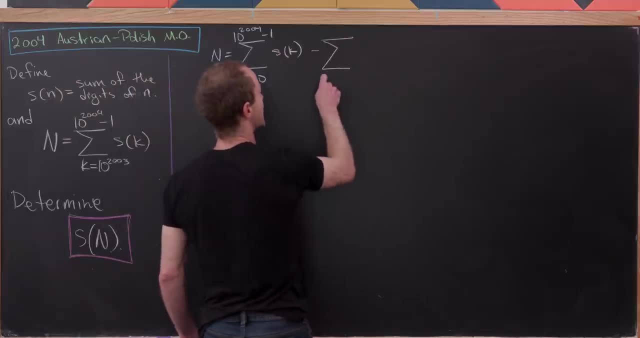 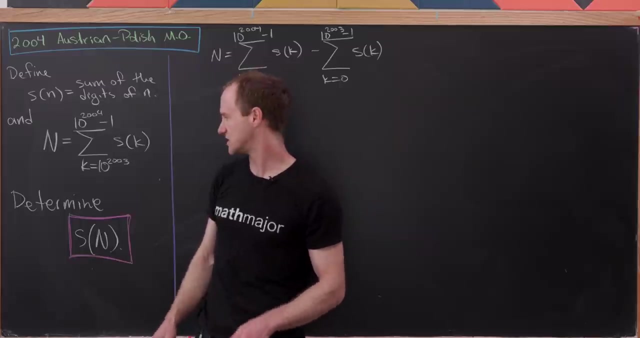 of k, The sum as k goes from 0 up to 10 to the 2003, minus 1 of s of k. So, of course, expressing it as this difference really just changes the starting point to this, k equals 10 to the 2003.. But it'll. 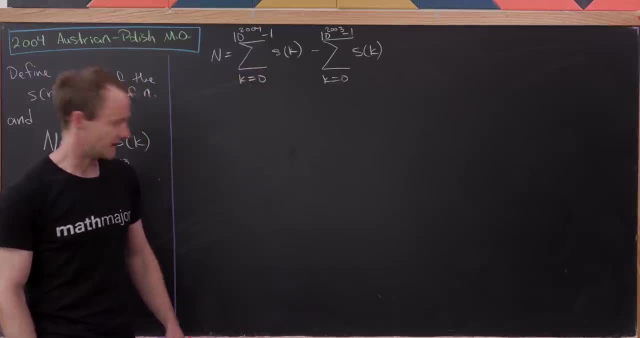 be a little bit easier to work with this. Okay, so now let's observe that this sum, as k, goes from 0 up to 10, to the 2003 minus 1 of s of k, So, of course, expressing it as this: 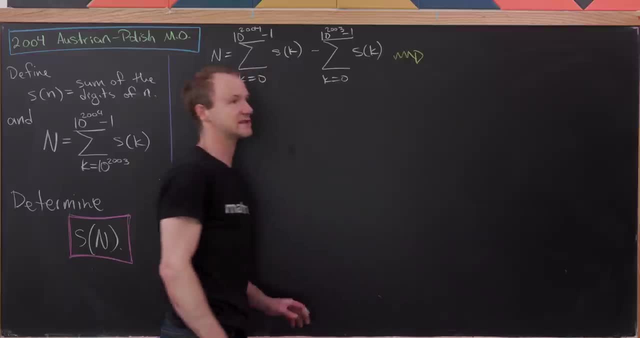 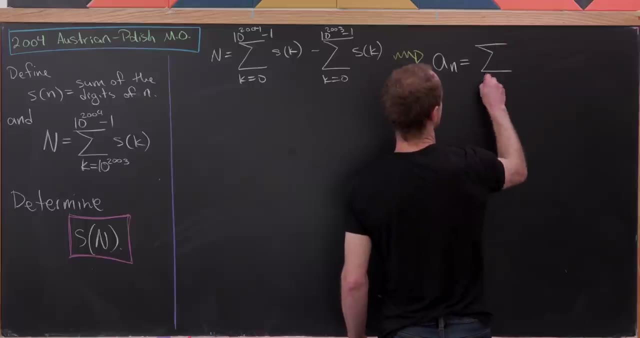 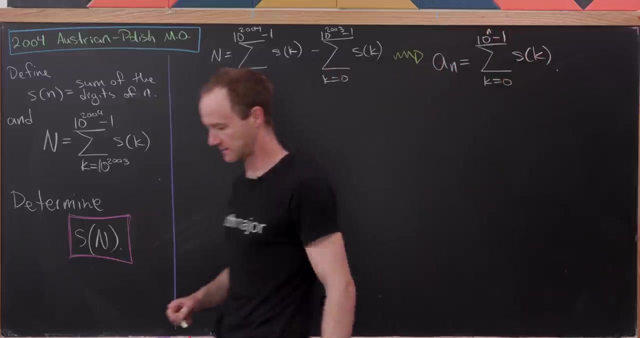 motivates us to look at the following sequence of numbers, And I'll call them a sub n. So there'll be a sub n which is equal to the sum as k goes from 0 to 10, to the n minus 1 of s of k. And, if we can, 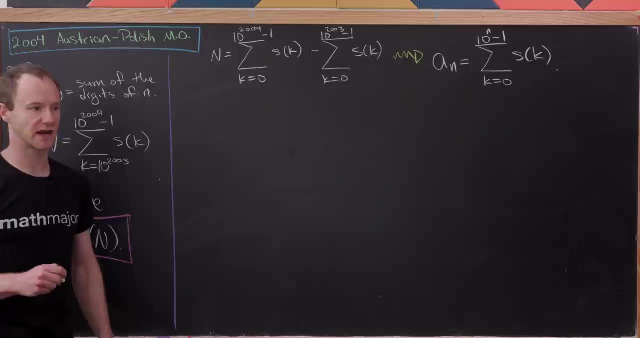 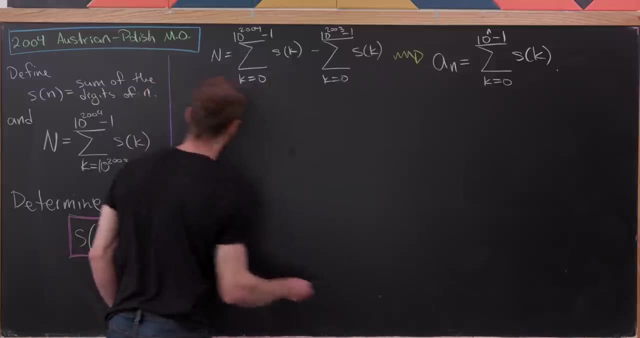 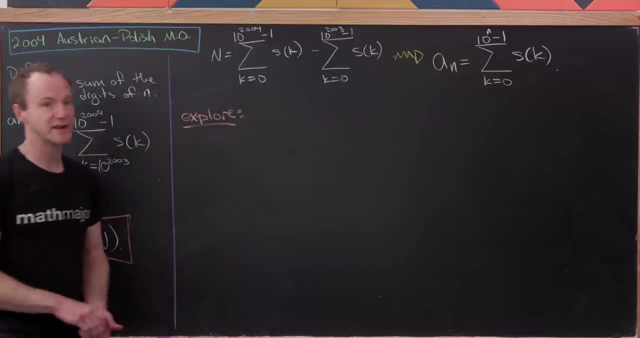 get a handle on what this sequence, a sub n, looks like. well then, well, we're essentially all set. So let's maybe explore the first couple of values of this sequence to see if we can come up with some sort of reasonable expectation for a closed form, And then perhaps we could prove that closed form. 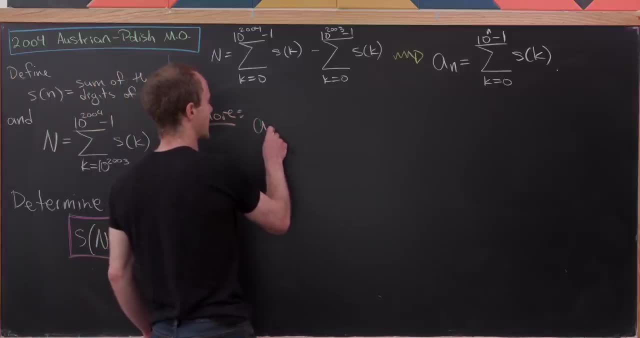 using induction. Okay, so let's observe that a sub 1,- well, that's going to be the sum, as k goes from 0 up to, well, 10, to the 1 minus 1, which is 9 of s of k. So let's observe that a sub 1,- well, that's going to be the sum as k goes from 0 up to, well, 10, to the 1 minus 1, which is 9 of s of k, And then perhaps we can come up with some sort of reasonable expectation. 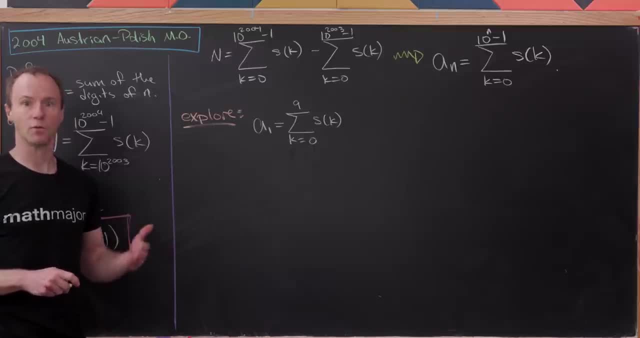 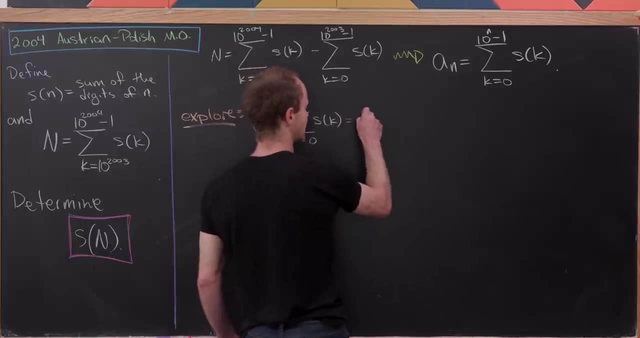 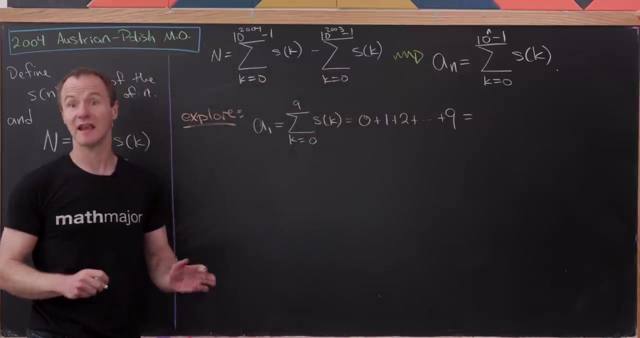 Notice that this is just the digit sum of some one-digit numbers. but the digit sum of one-digit numbers are simply those one-digit numbers. So here we're going to get that this is equal to 0 plus 1 plus 2, ending at 9.. But that's really the ninth triangular number And there's a closed form. 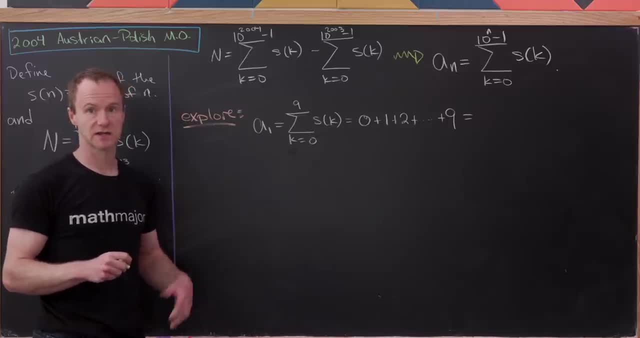 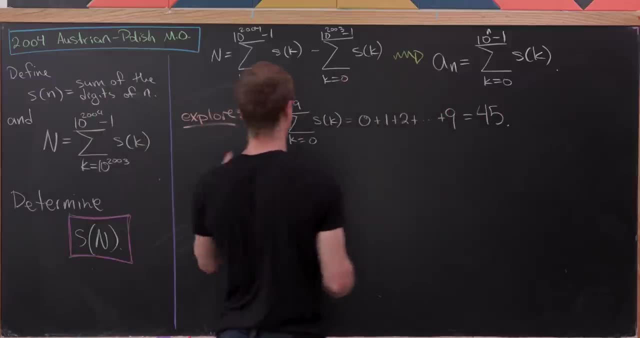 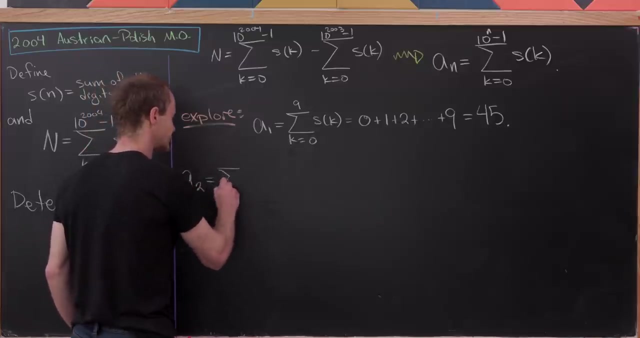 for triangular numbers. So this is going to be 9 times 9 plus 1 over 2.. In other words, 9 times 5 aka 45. So we've got a sub 1 is equal to 45.. Now let's look at a sub 2.. So that's going to be the. 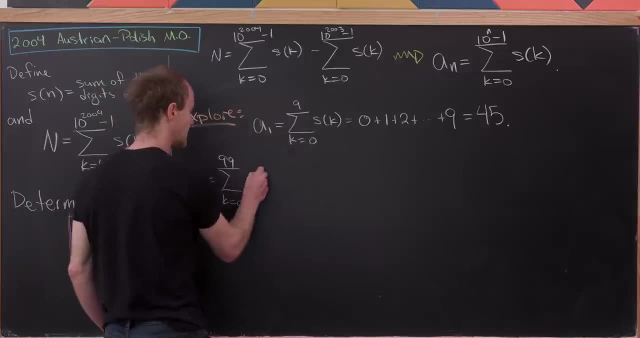 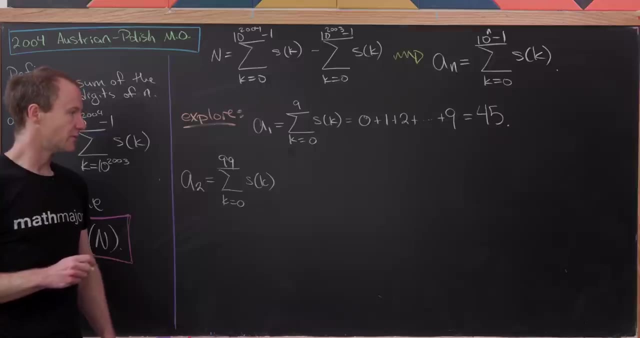 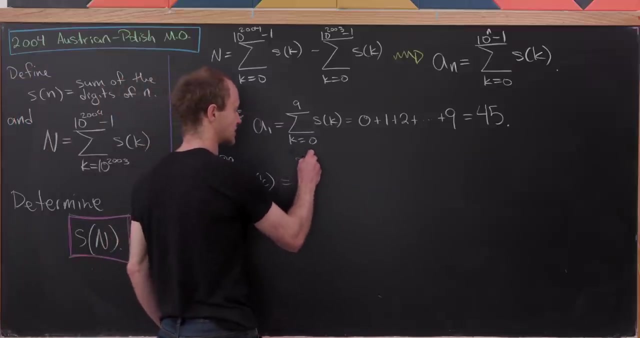 sum as k goes from 0 to 99 of s of k. Now this may seem like pretty hard to work with, but if we break it into chunks of 10 it won't be so bad. So I'll just write out those chunks of 10.. So we'll. 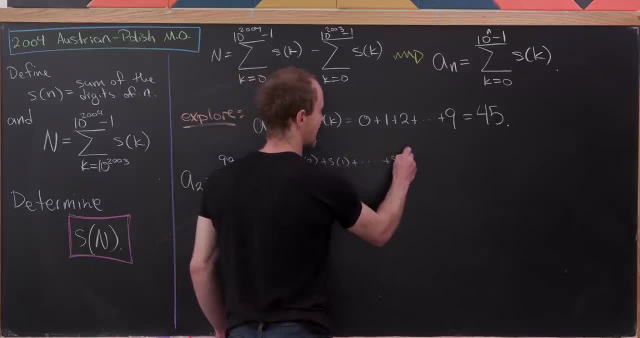 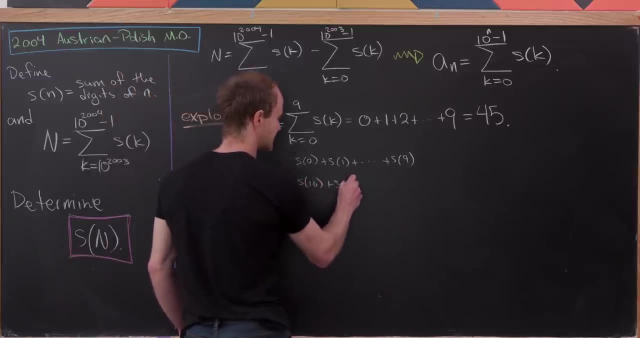 have s of 0 plus s of 1 all the way up to s of 9.. So those are the one digit parts, And then we'll have s of 10 plus s of 11 all the way up to s of 19.. So those will be the parts, obviously between 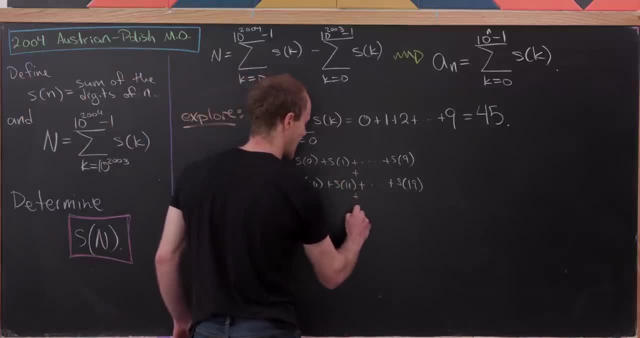 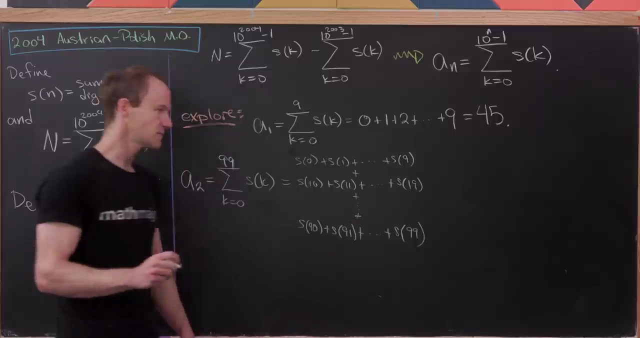 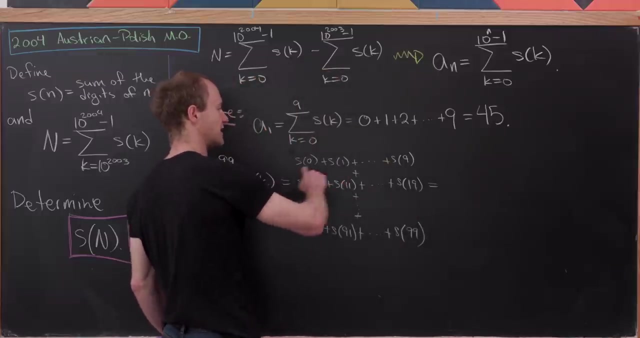 10 and 19.. And then let's see. the last bit will be s of 91, or sorry, 90 plus s of 91, ending At s of 99.. Okay, great, But now we can calculate each of these pretty easily. Observe that well. 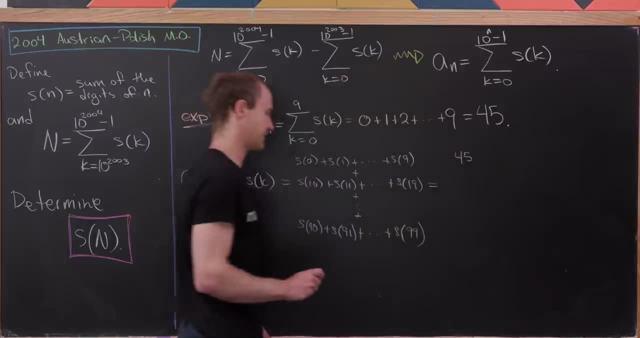 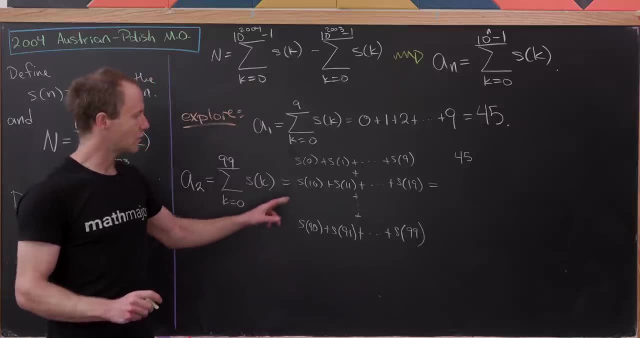 this first line is simply equal to 45. And then this second line: well, we're going to get 45 from everything in the ones digit. And then, well, observe that we also have a 1 for everything in the tens digit, but we have exactly 10 ones. 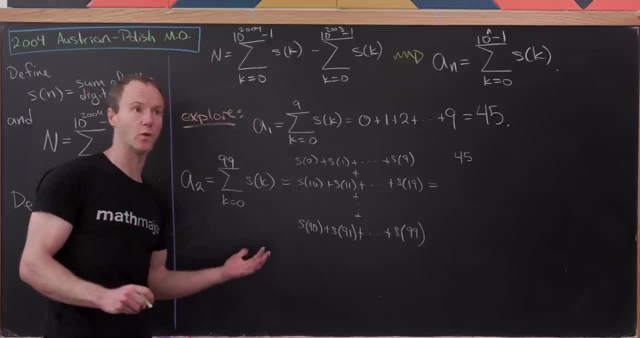 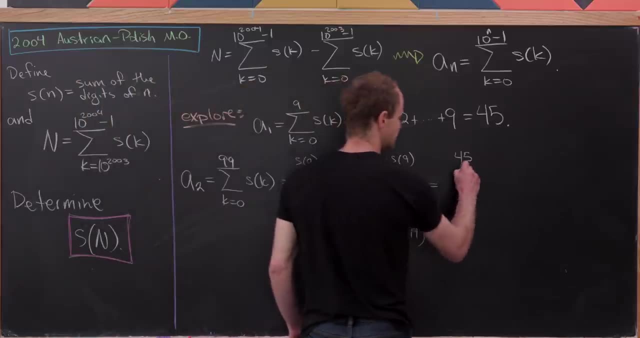 So that's going to give us, well, 45 for the sum of the ones digits, And then 10 times 1, in other words 10 for the sum of the tens digits. So that's going to be: we have plus 45 plus 10.. And then for the 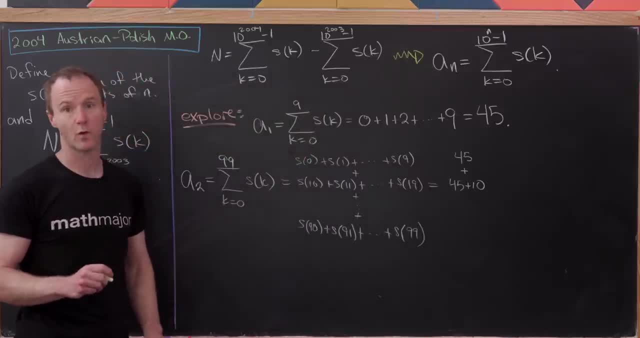 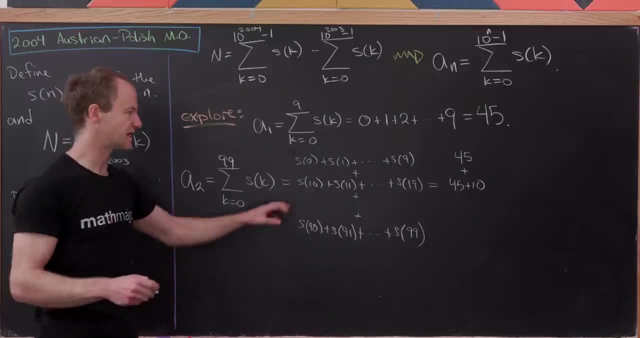 next bit. well, we're going to have another 45 for the sum of the ones digits, And then we'll have, well, 10 times 2 for the sum of the ones digits, because the next line is going to be all of the 20s. 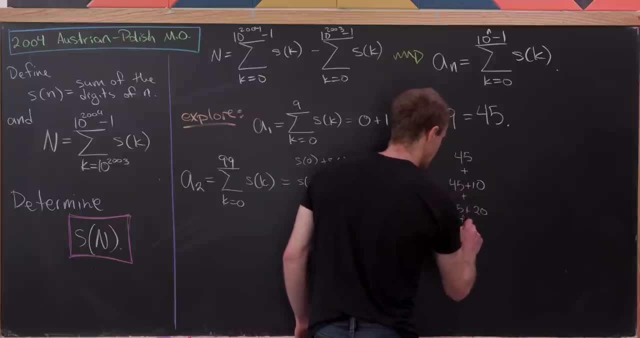 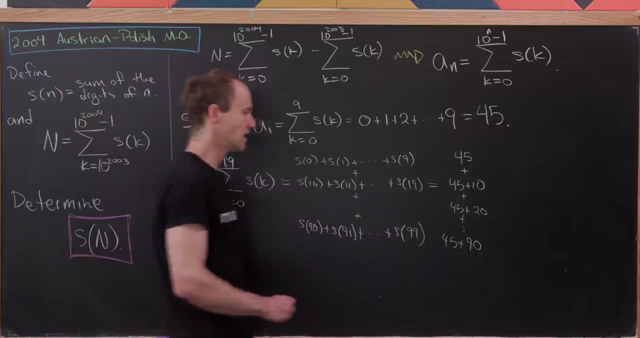 And then we'll have: this is plus 45, plus 20.. And then this is all the way up to 45. plus 90 is this last line. But let's see, how many of these 45s do we have? Well, we have 10 lines here, so that's going to. 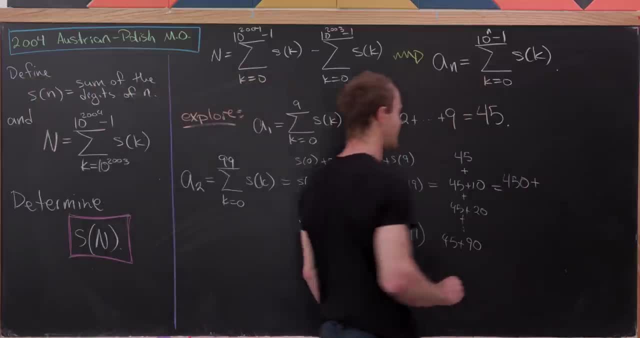 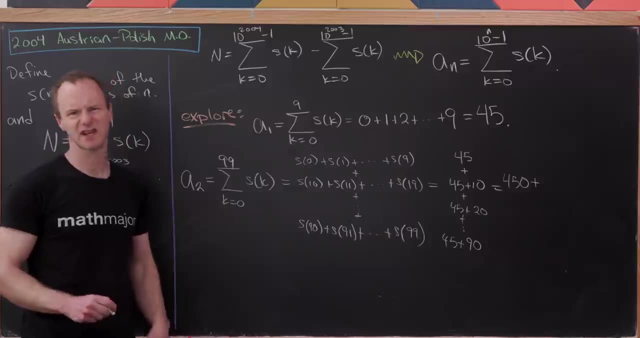 add up to 450. And then after that we have 10 plus 20, plus 30 plus 40, all the way up to plus 90. But that's just going to be 10 times the triangular number that we saw right here. 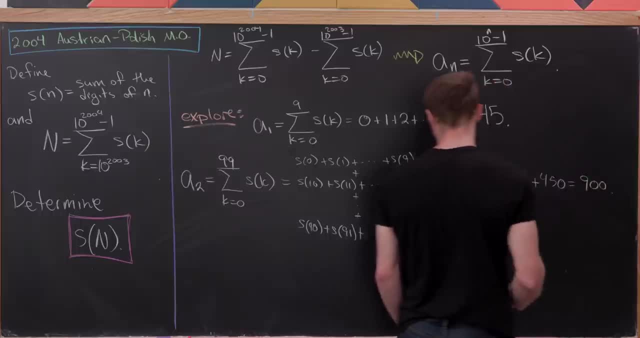 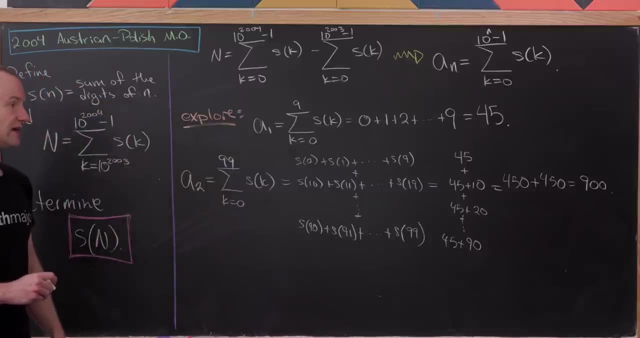 In other words 450 again. Well, that's going to add up to 900.. Okay, so we've got 45 for a sub 1.. We have 900 for a sub 2. And then for a sub 3.. Well, we can play this whole game again. But now, 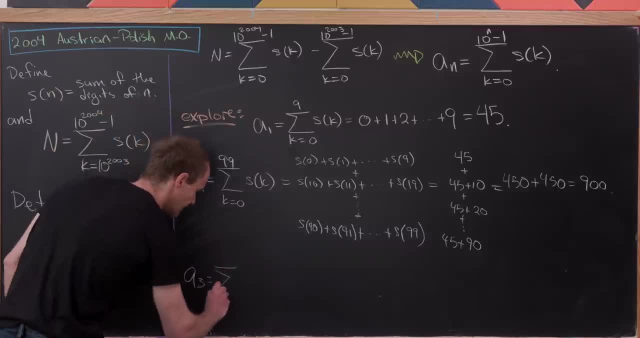 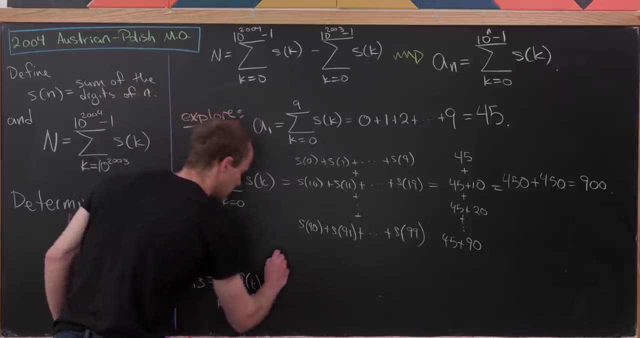 we'll break it into chunks of hundreds. So we've got this sum as k goes from 0 to 999 of s of k. And Well, we'll have s of 0 plus all the way up to s of 99. And then this is going to go all the way. 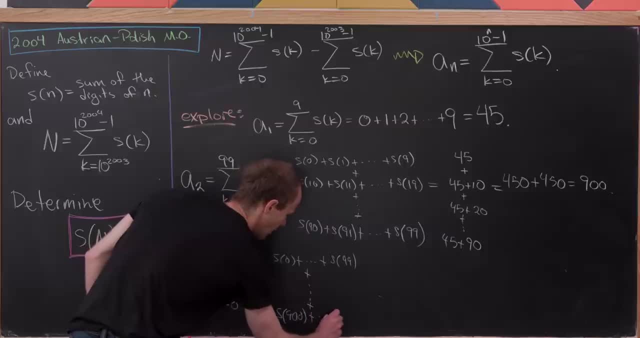 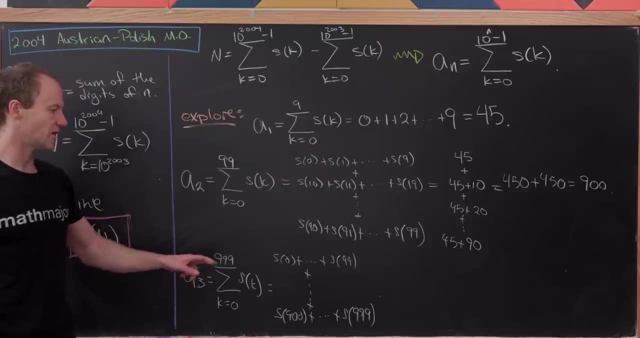 down to s of 900, all the way up to s of 999.. And then, well, we know that this first line is equal to 900, just as before. The second line is going to be well, 100 plus 900, and so on and so forth. 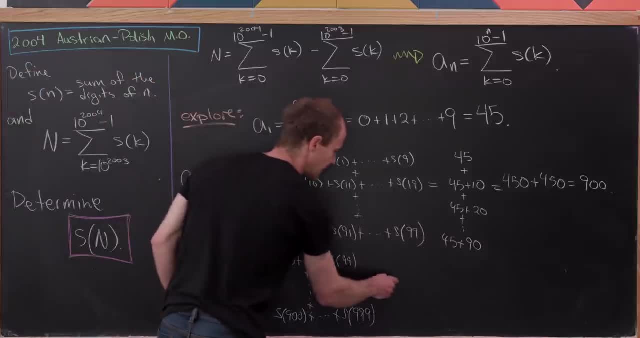 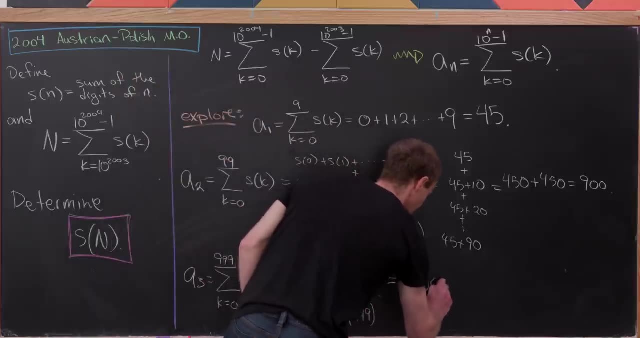 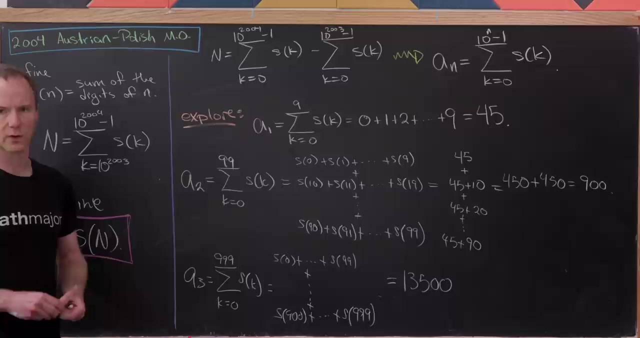 Just like we did up here. So in the end- and maybe I'll let you do all of the arithmetic- What you'll see here is we get the number 1, 3, 5, 0, 0.. But of course we'd like to have some sort of nice formula that ties this into the index. 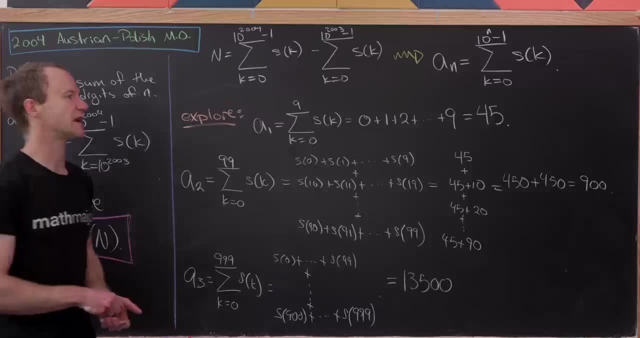 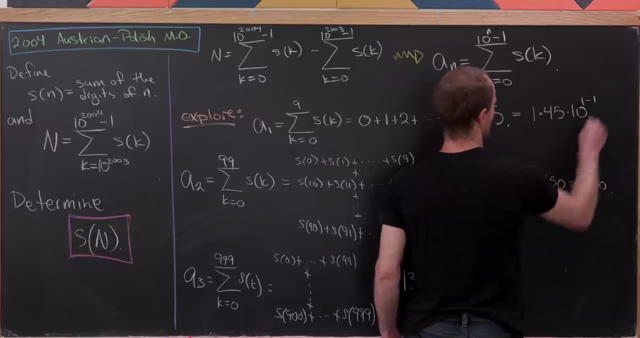 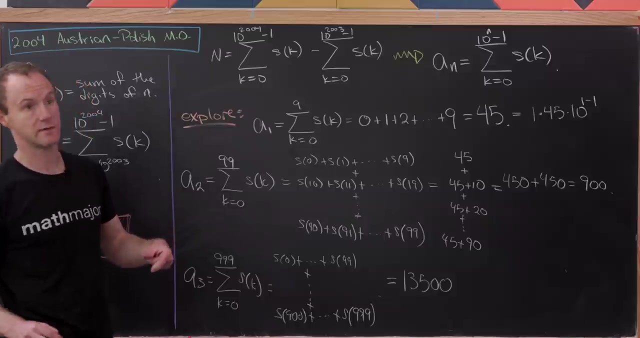 that we see. So, looking at this a little bit more carefully, observe that this is equal to 1 times 45 times 10 to the 1. Minus 1.. So here I've got 1 for my index, a sub 1, and then 10 to the 1 minus 1, again for my index, a sub 1.. 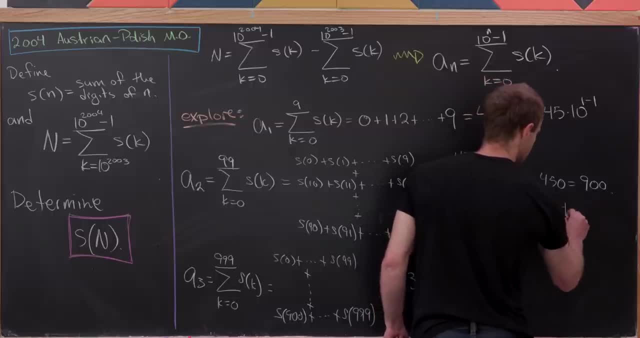 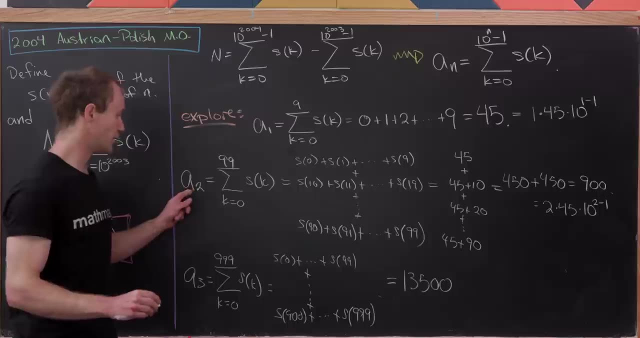 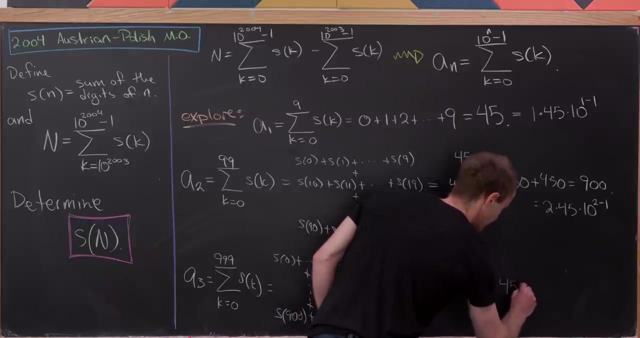 Whereas this thing right here is going to be 2 times 45 times 10 to the 2 minus 1.. So, again, we work that 2 in there And then, well, you can check that this number is equal to 3 times 45 times 10 to the. 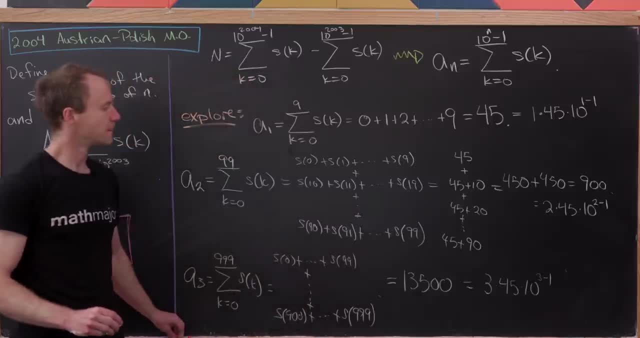 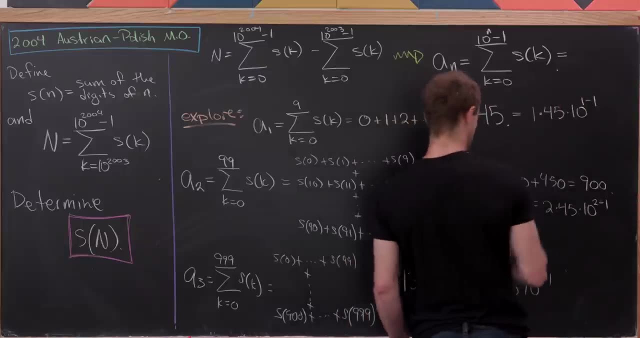 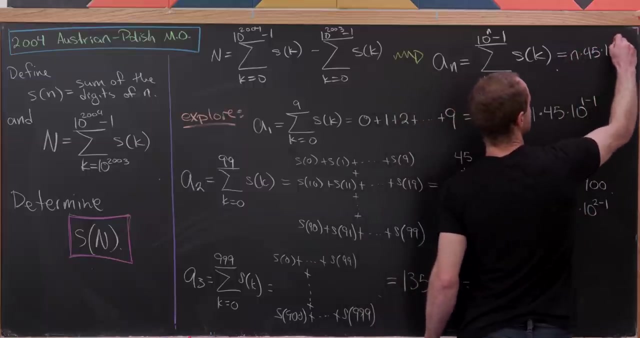 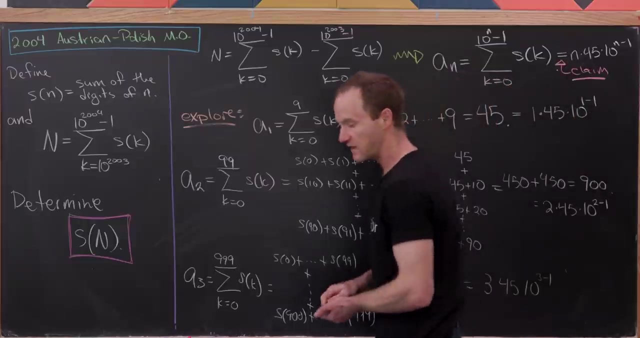 3 minus 1.. So well, what does it look like? Well, it looks like this should be equal to n times 45 times 10, to the n minus 1.. So maybe we'll make this our claim and then perhaps, on the next board, we'll start proving that claim by induction. 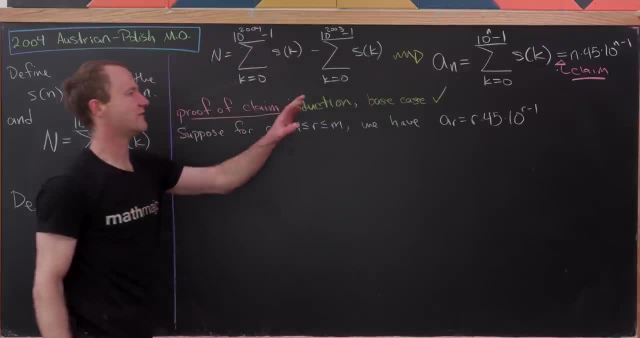 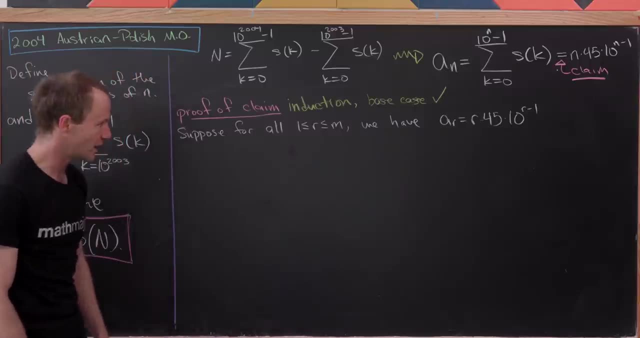 OK, So jumping into our proof by induction of our claim that a sub n is equal to n times 45 times 10 to the n minus 1.. Well, we need to obviously start with a base case, but the base case is done by all of the exploration on the last board. 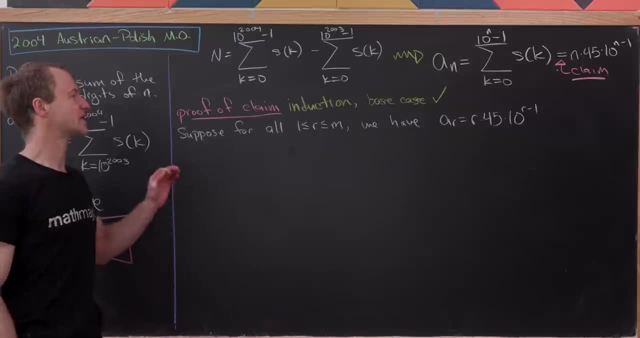 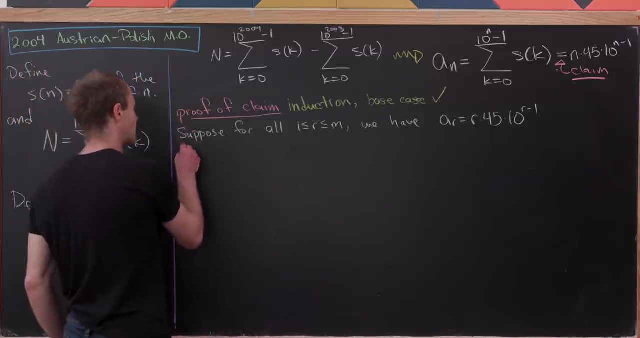 So now we simply need to make an induction hypothesis, And in this case it'll be a strong induction hypothesis. So that means, for all R between 1 and M, we'll assume that a sub r is equal to r times 45 times 10, to the r minus 1, and then we'll consider: 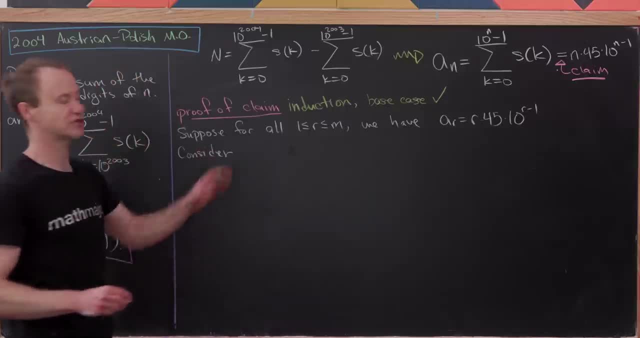 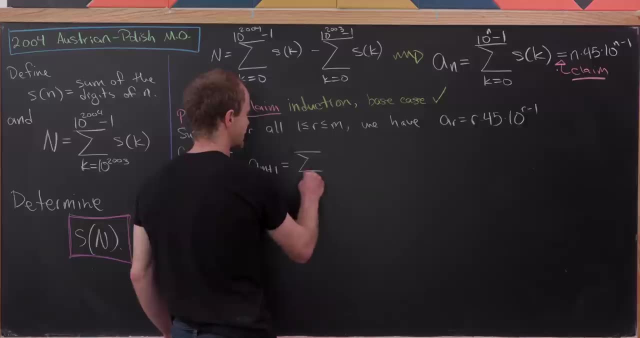 the next case, the unproven case, which is the m plus first case. so let's do that. we have a sub m plus 1, so by definition that's the sum as k goes from 0 up to 10 to the m plus 1 minus 1 of. 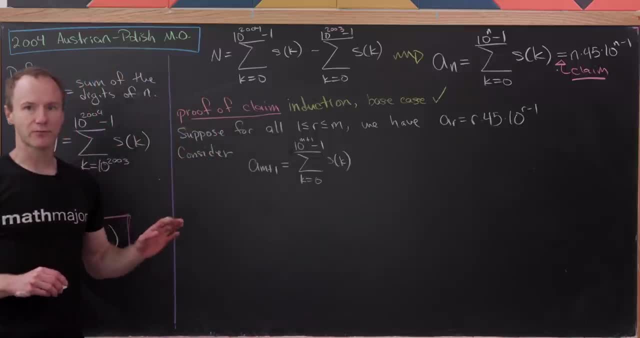 s of k, but now i'm going to break this into 10 parts, just as we broke our a sub 2 and our a sub 3 pieces into 10 parts as well, and it's going to look like this: so we're going to have the sum. 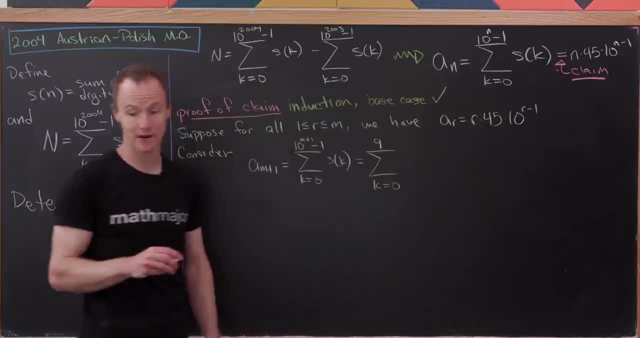 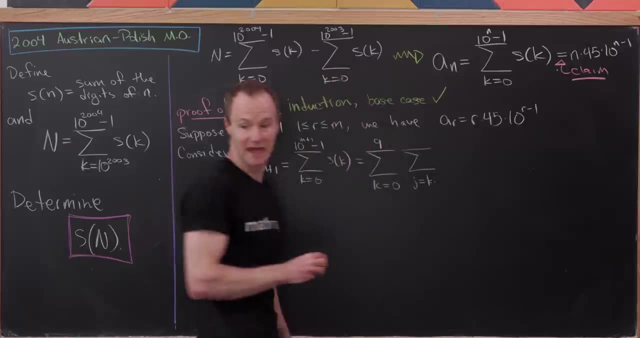 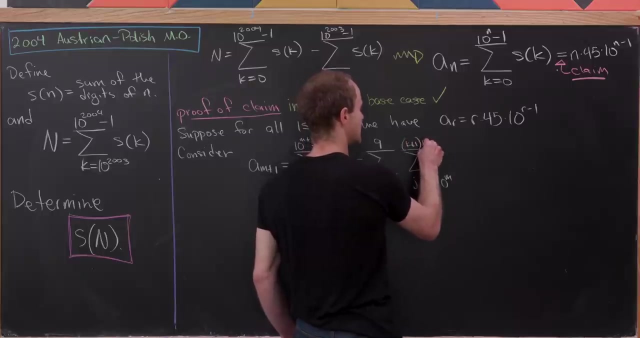 as k goes from 0 to 9. so those are our 10 parts, and then inside of that we'll have the sum as j goes from k times 10 to the m, all the way up to k plus 1 times 10 to the m minus 1. so this is like going from 0 to 9. 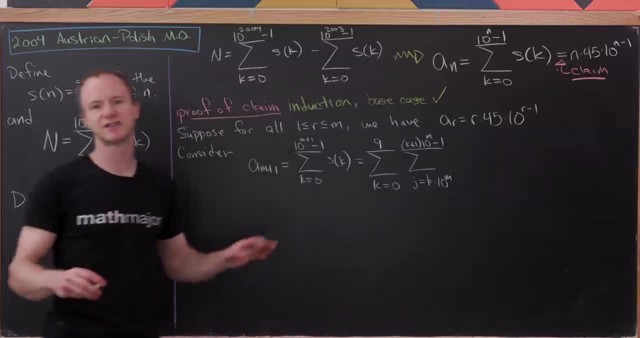 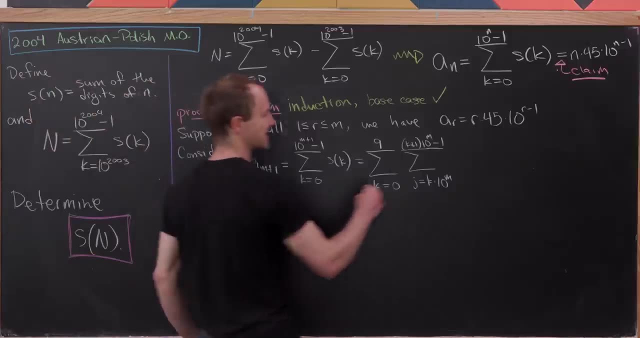 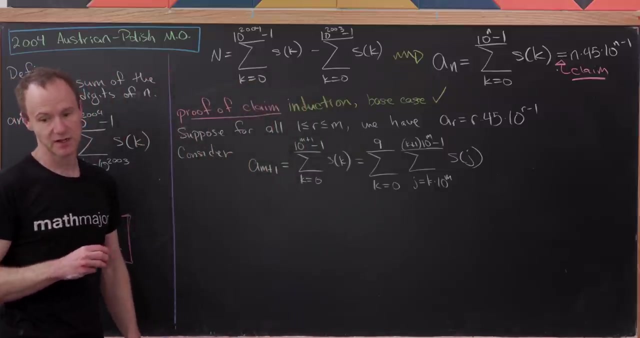 10 to 19, 20 to 29 and so on and so forth. in that a sub 2 case, okay, so now, uh, oh, i forgot this. i've got my s sub j here now next up. what i'd like to do is re-index that inner sum so that it starts at: 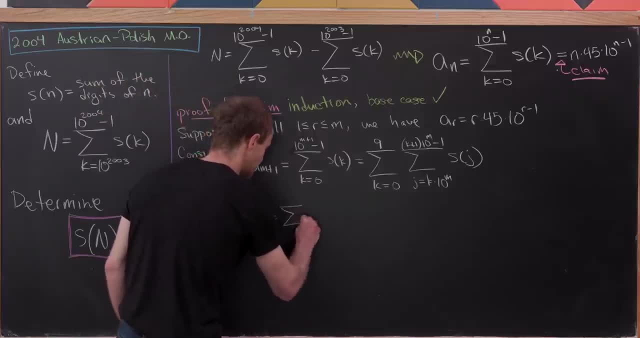 zero. so let's do that again. so we're going to have the sum as k plus 1 times 10 to the m minus 1. let's do that, so my outer sum is staying the same. my sum is k goes from 0 to 9, and then, if i 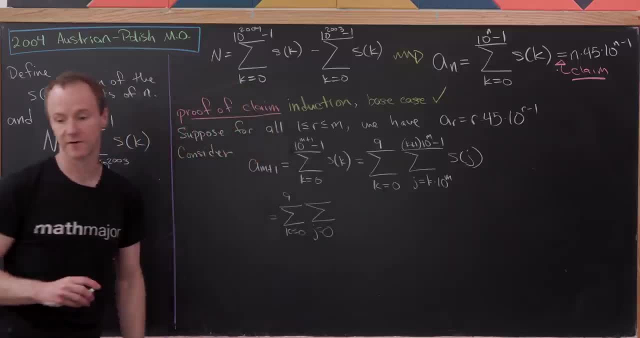 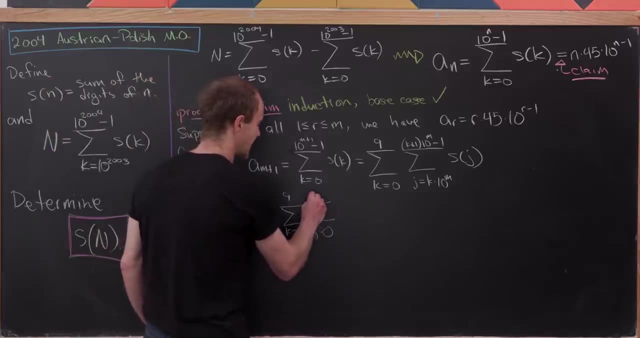 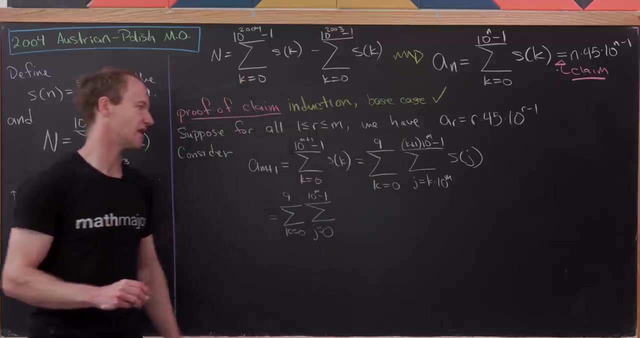 re-index. so it starts at zero. i'll have j going from zero up to. let's see that's in fact going to be equal to 10, to the m minus 1. so you can check that pretty easily just by the difference of those two maybe indices, the upper and lower bound, and then we'll have s. 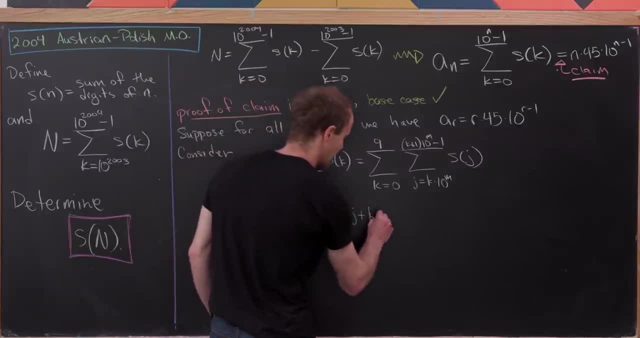 of j, and then we'll have j minus 1, and then we'll have j minus 1, and then we'll have j minus 1, k plus k times 10 to the m. but now let's observe that we can take this s of j plus k times 10 to the. 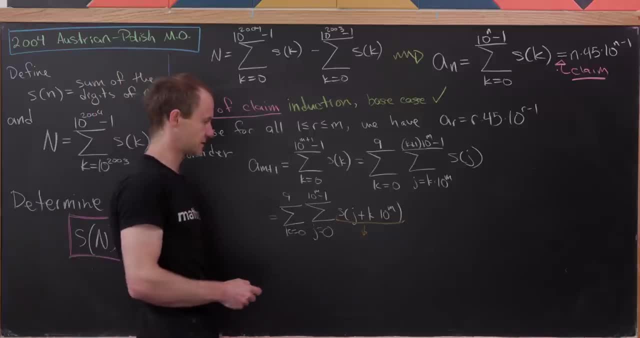 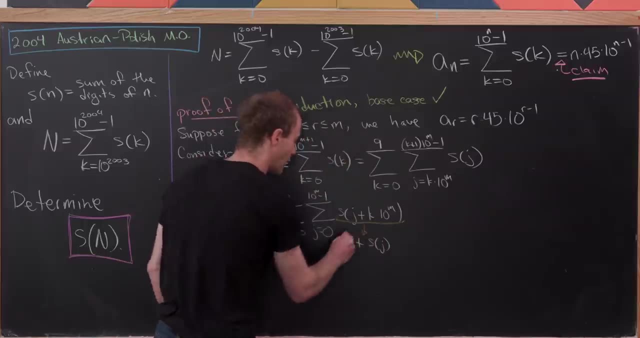 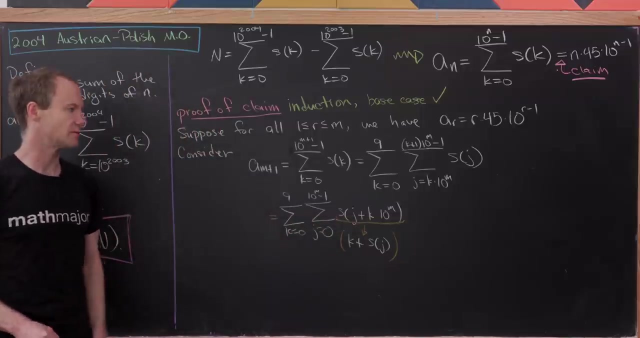 m and rewrite it as follows: so this is going to be equal to k plus s of j. and well, why is that? well, that's because this k is the leftmost term, yeah, the leftmost term, in the you know expansion of the number. but then the j is playing the role. 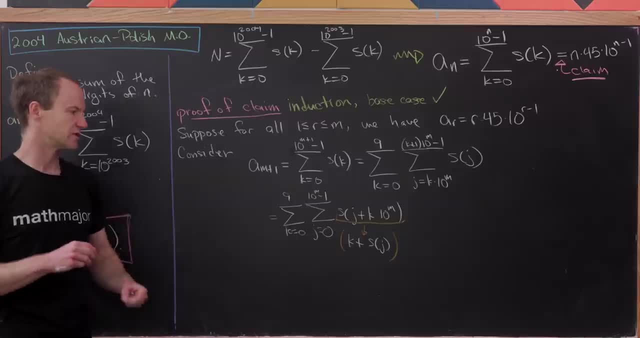 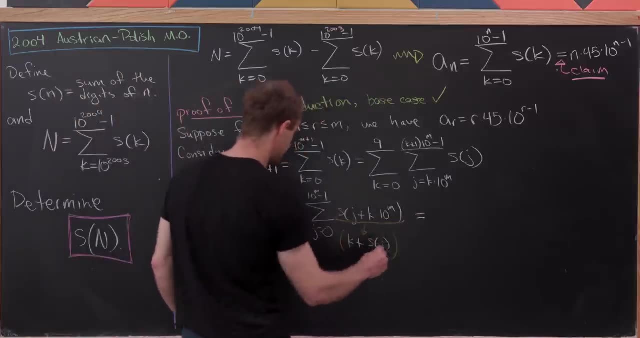 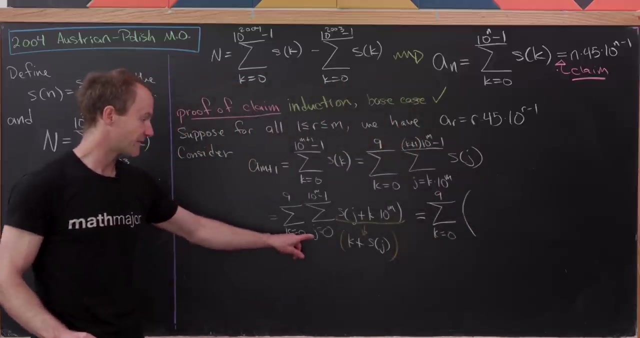 of all of the rest of the terms, so those are independent of each other. and now, well, we can sum this inner bit. so observe, well, we still have this sum as k goes from 0 to 9. and then summing k from j equals 0 to 10, to the m minus 1. that's just summing a constant. 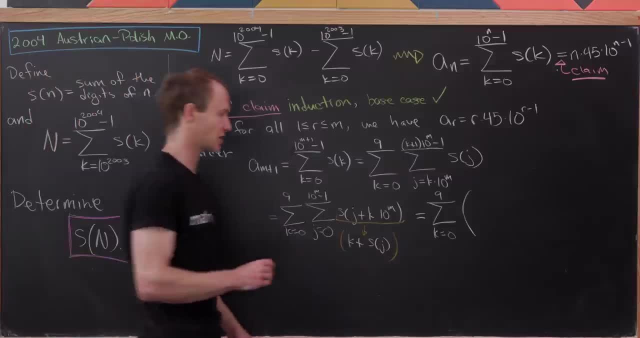 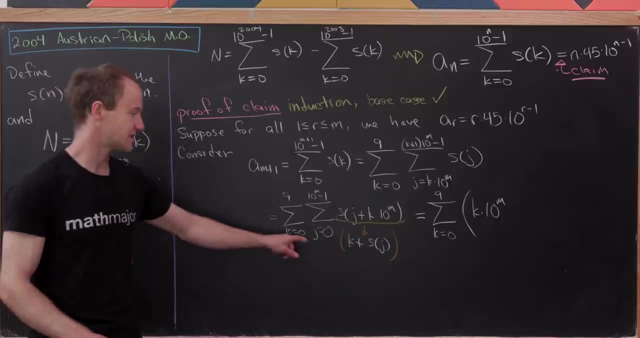 for how many terms? well, 10 to the m terms. so that's going to give us k times 10 to the m. so that's from the k term, and then summing s of j from j, from 0 to 10 to the m minus 1, that's our. 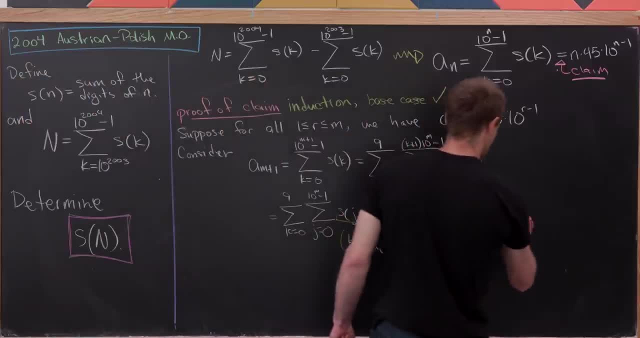 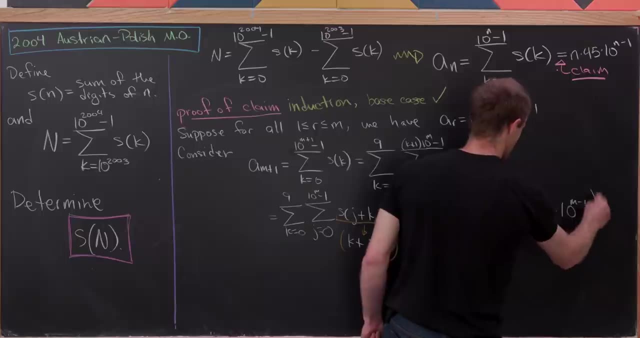 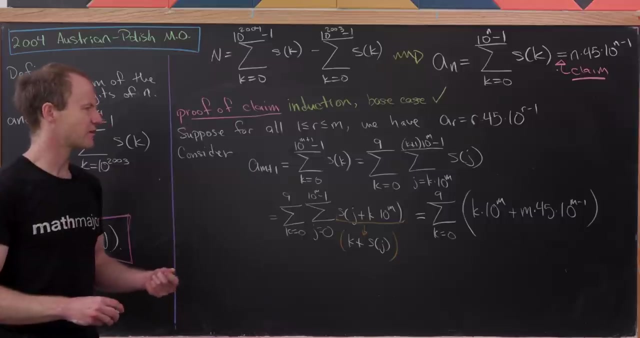 induction hypothesis. so that's going to, in fact, be equal to m times 45 times 10, to the m minus 1. okay, so i think that's looking pretty good. so we're going to sum this in here and we're going to look at this a little bit more carefully. maybe we didn't need a strong induction hypothesis. 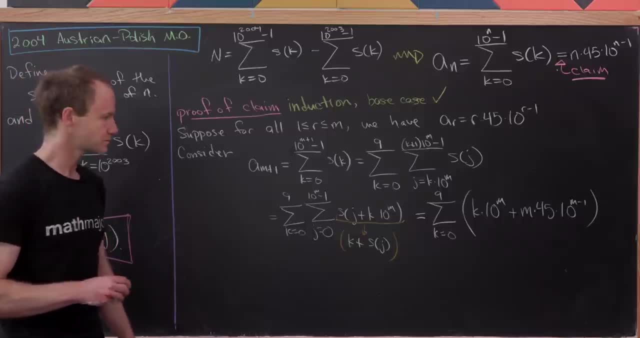 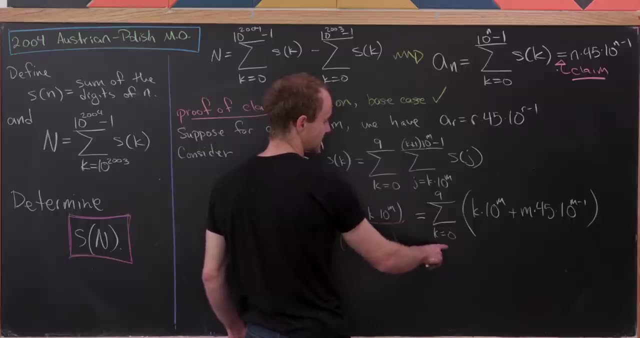 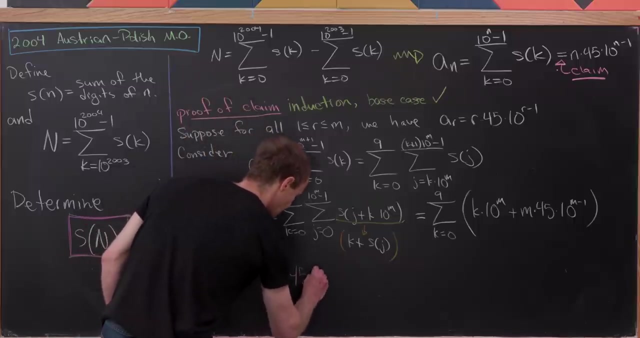 that being said, it's okay to write one down, okay. so now, well, observe that this is simply 10 to the m times a triangular number, this sum of 0 up to 9. that's this first term, but we already know that that's 45. so here we get 45 times 10 to the m, so we're adding this term to itself 10 times. 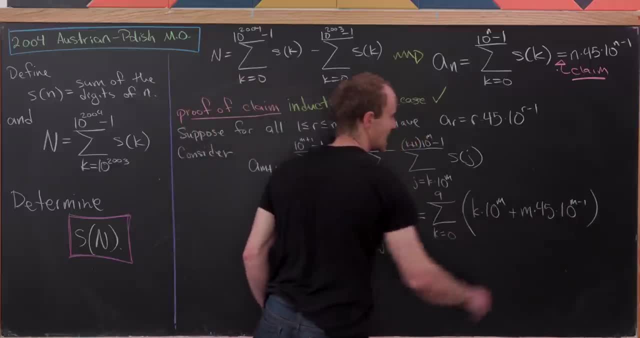 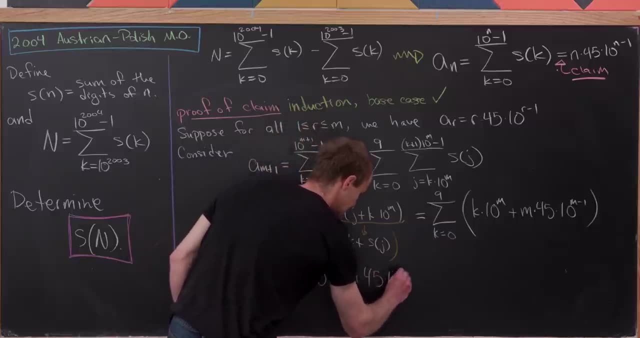 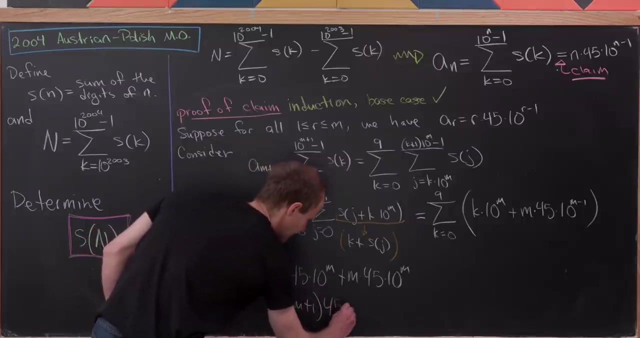 but that'll just give us 10 times that term, which will bump that m minus 1 exponent up to an m exponent. so here we have m times 45 times 10 to the m. but now, oh well, we can add those together and we'll get m plus 1 times 45 times 10 to the m. but that's exactly the shape that we need. 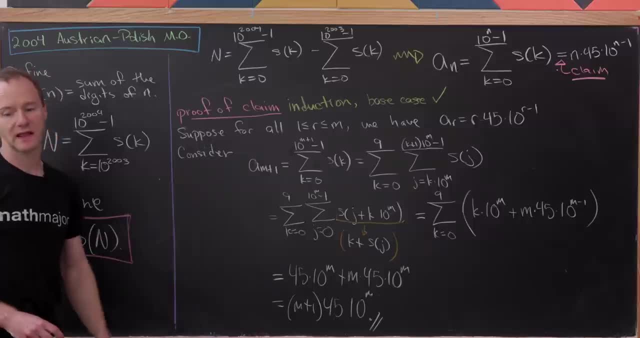 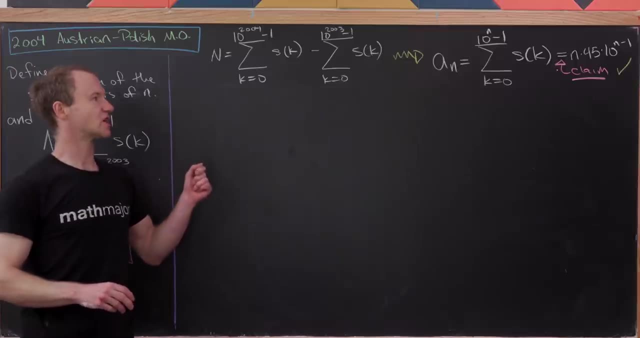 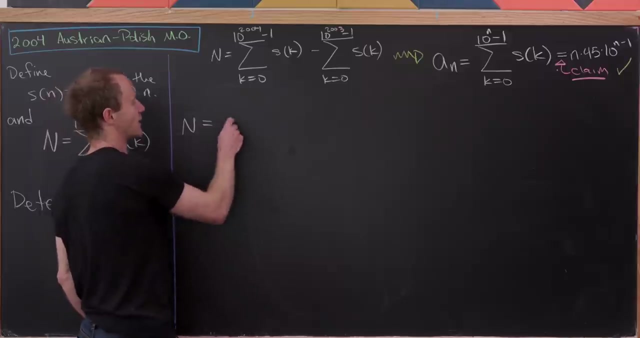 in order. well, for the proof of that claim to be done, okay, so now let's apply this claim to finish everything off. okay, so we just finished off the close form for our sequence, a sub n, and now let's observe that, in the language of a sub n, we know our capital n is a sub 2004. 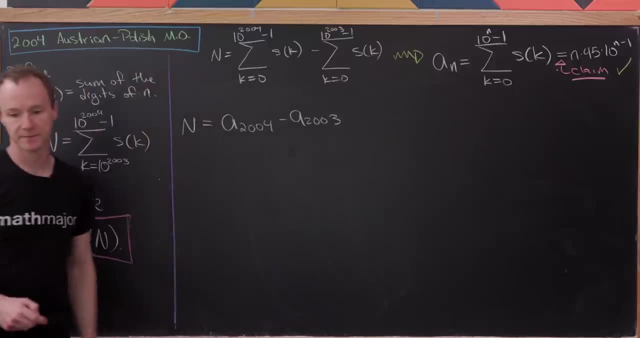 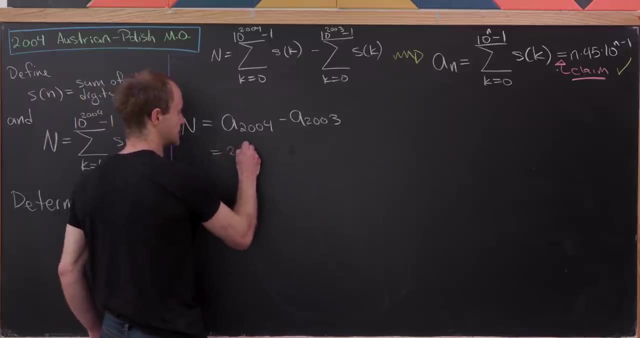 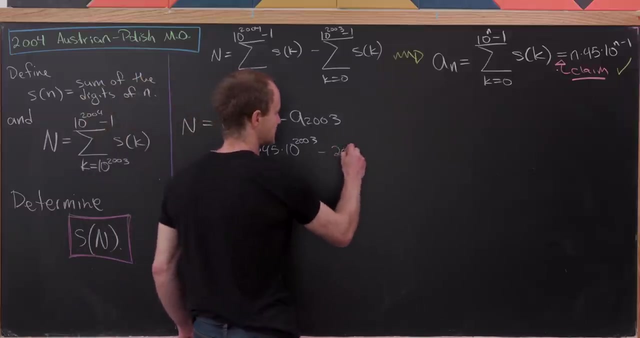 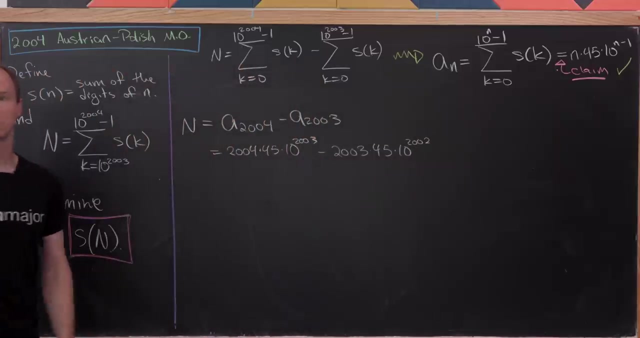 minus a sub 2003. so now, putting in the value that we proved via that claim, we know that this is going to be 2004 times 45 times 10 to the 2003, and then minus 2003 times 45 times 10 to the 2002.. So let's take out a greatest common factor, which? 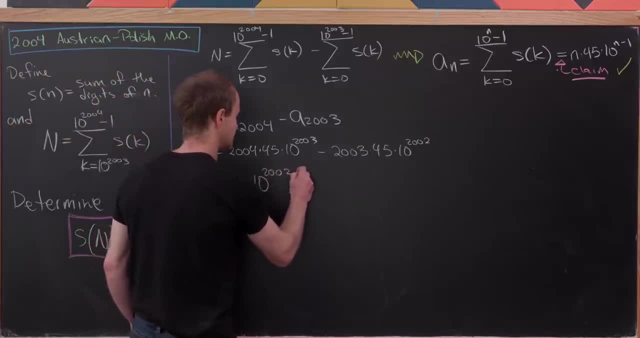 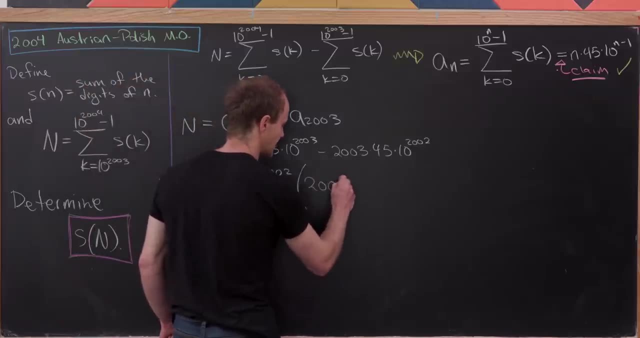 in this case, is going to be 45 times 10 to the 2002, and that's going to leave us with 2004 times 10.. In other words, 2004- well, sorry, 20,040 minus 2003.. Now, of course, this is a simple arithmetic. 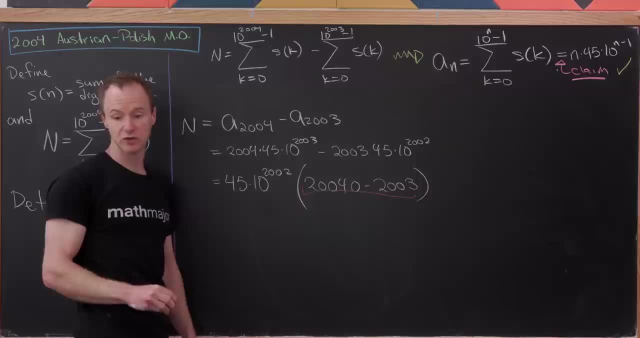 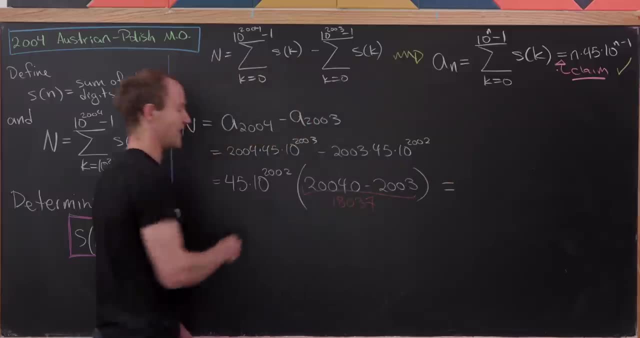 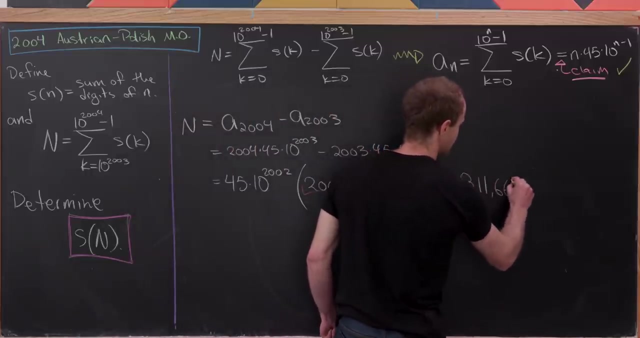 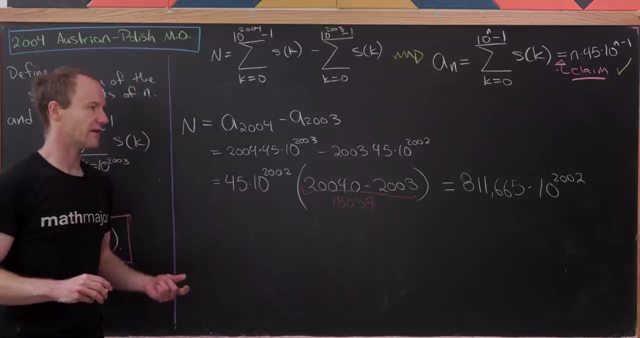 problem right here. We can subtract those two numbers and we'll get 18,037, and then multiply that into 45 and we'll get 811,610.. So we have our number. n is well that 811,665 times 10 to the 2002. but 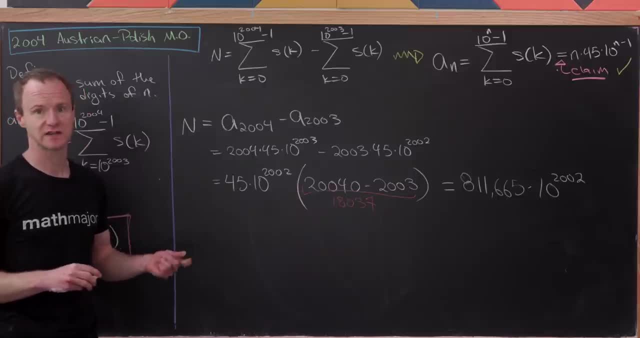 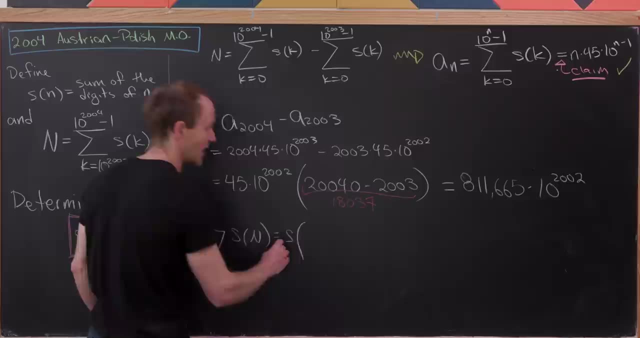 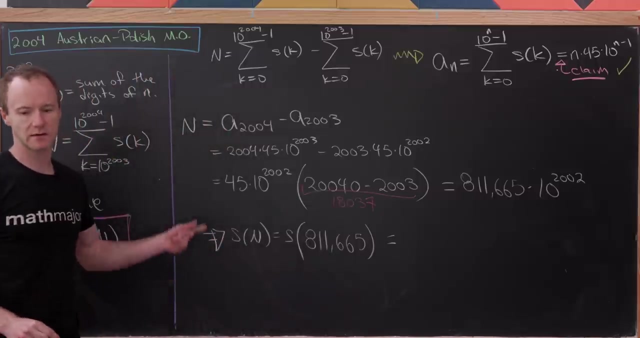 the multiplication by 2010 to the 2002 doesn't change the digits sum. So in fact s of n is simply s of this: 811,665. eight hundred and eleven thousand six six five, but of course that's simply going to be eight.